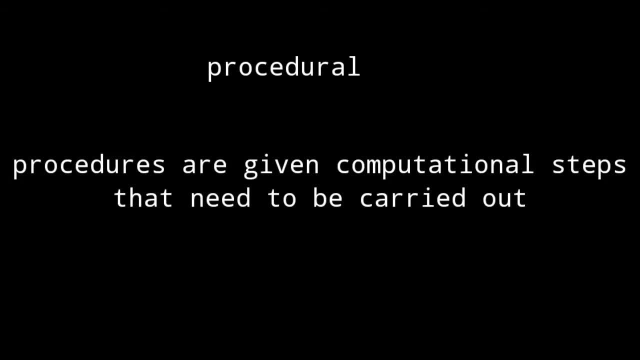 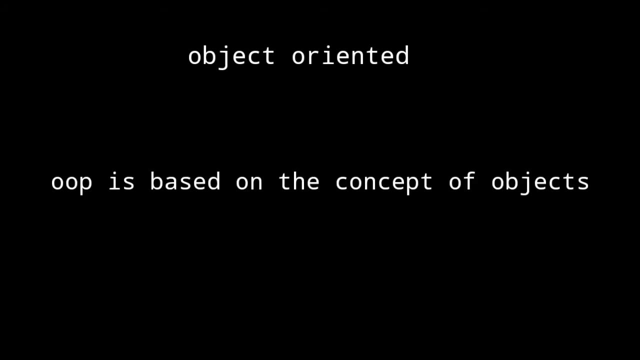 type is made of things called procedures, and procedures are given computational steps that need to be carried out. any procedure can be called at any time during execution. now we come to object oriented. one of the most famous OOP or object oriented programming is based on the concept of objects. now objects. 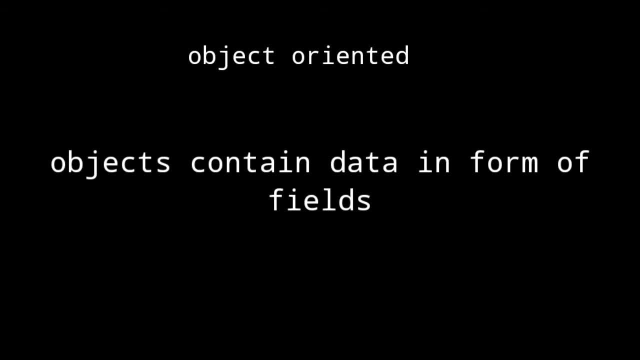 contain data in form of fields now, while code is stored in form of procedures. the field is basically a unit of database, you know, like a field in our DBMS. now most OOPs use inheritance and hence have classes in them. this in terms, add flexibility and extent, extensibility, and best examples would be: 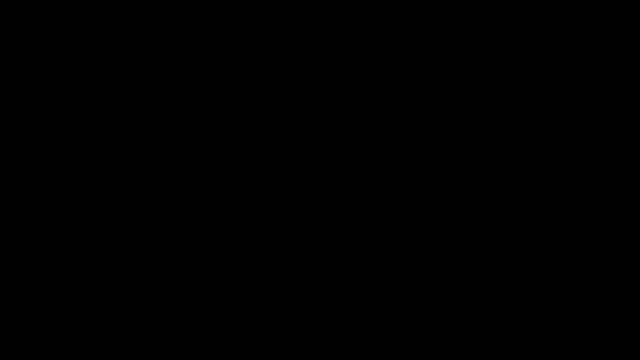 Java, Ruby and Python. now we come to declaration programming. the declarative programming is one in which we give logic of computation, but not the control flow. now, what is control flow? now? it is an order in which statements, instructions and functions are executed. basically, we tell what we want to get, but not how to get it. now you can think it as your parent. 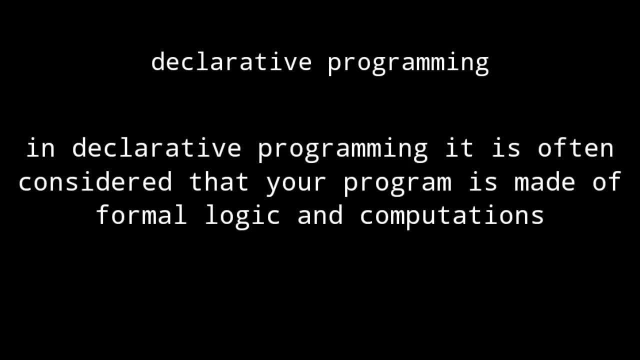 asking a child for marks. now, in declarative programming, it is often conceded that your program will not be able to get what you want. it to get what you want, and that's why you have to make it your way, and that's what it's about. why is it called a declarative programming? let's talk about that in a 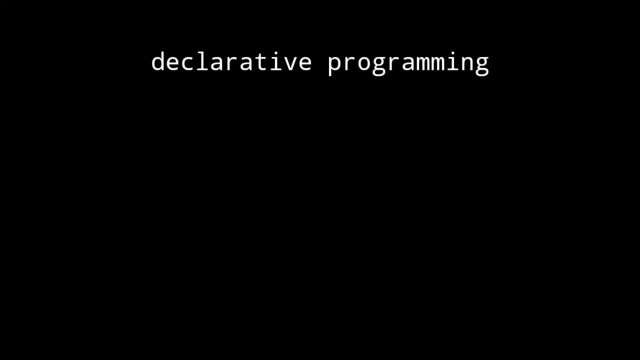 more general way, it's a form of logic where the program is made of formal logic and computation. formal logic is logic defined by a set of rules and syntaxes, and declarative programming is greatly used in writing, parallel programs or parallelism. the best example of declarative programming would be SQL. 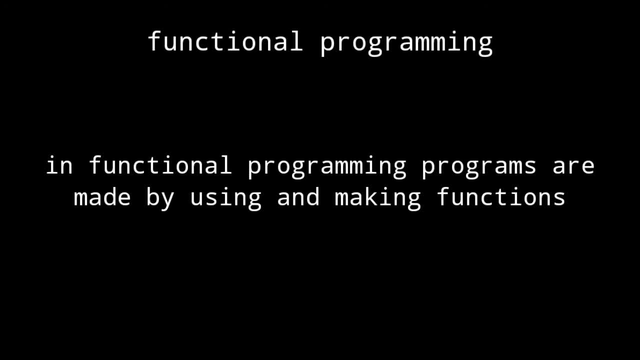 prologue: data log and Haskell. now we come to functional programming. now Functions. In this paradigm, functions are trees of expression that return a value. Functions are first-class citizens of this paradigm, which means they support all operations that other entities support. In this paradigm, functions can be bound to names returned from. 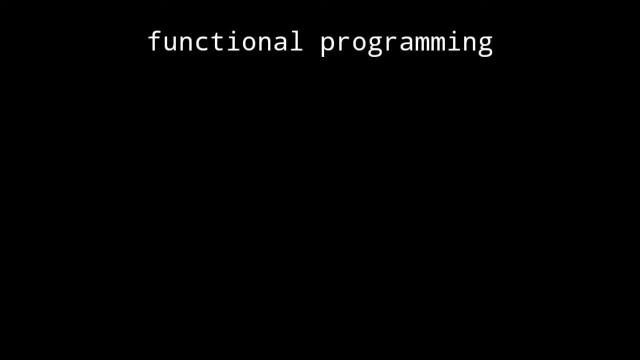 other functions or parsed as arguments, They behave like other datatypes. Many a times it is also treated as a purely functional programming, in which functions are treated as pure mathematical or deterministic functions. Functional programming is based over lambda calculus. Lambda calculus is a system of computation based on functions only, Although you don't. 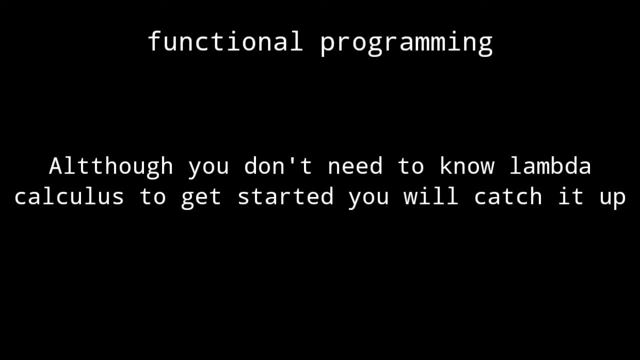 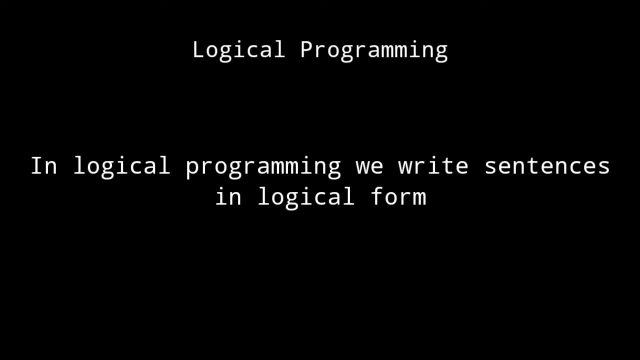 need to know lambda calculus to get started. you will catch it up. Some better examples: Haskell and ruby. Now we come to logical programming. Logical programming is based on formal logic. We know about it Now. in logical programming we write sentences in. 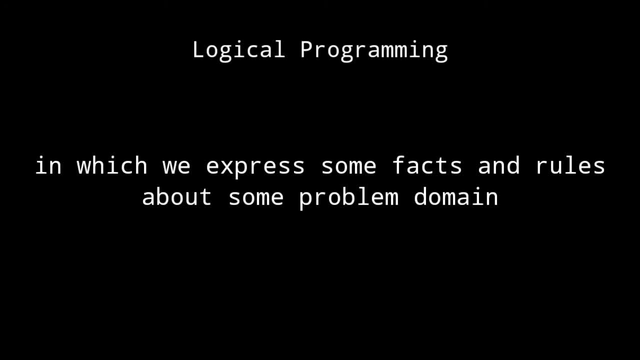 logical form in which we express some facts and rules about some problem domain. Best examples would be prologue and datalogue. In them we define rules and clauses- h, colon, b1, and like that. In them, h is the head of the rule and b1, and bn is the body. They are executed by proof. 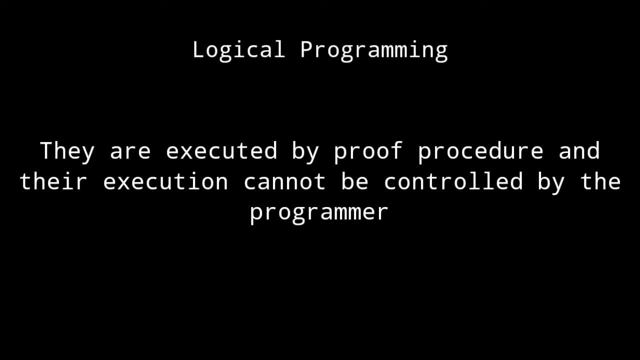 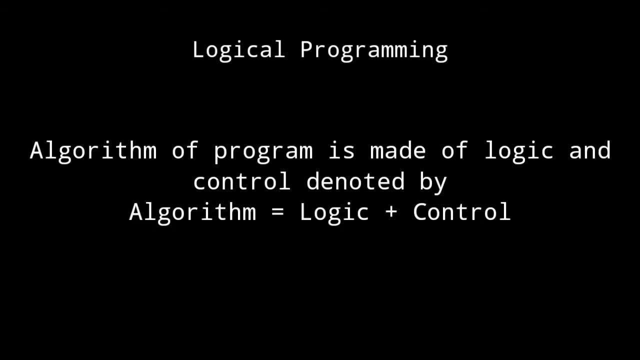 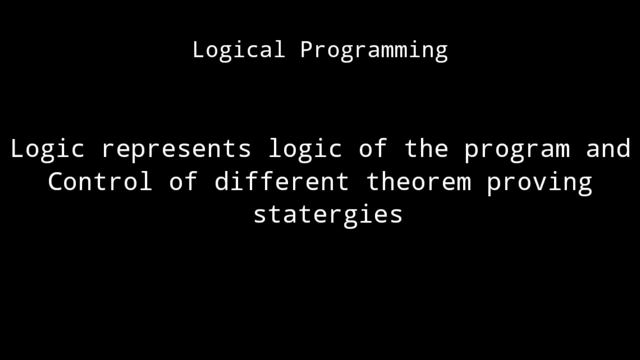 procedure and the execution cannot be controlled by the programmer. Now, a very basic concept of it is the logic and control. Algorithm of a program is made by logic and control Denoted by algorithm is equal to logic plus control. Logic represents the logic of the program and control 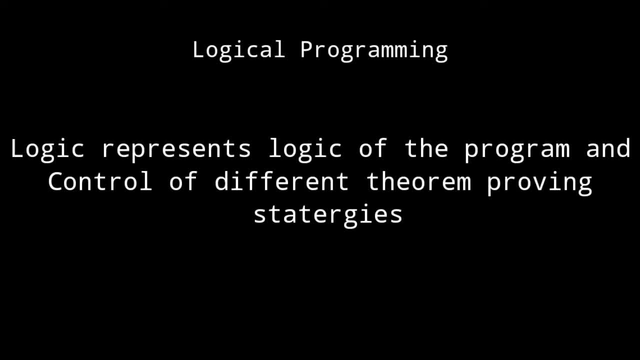 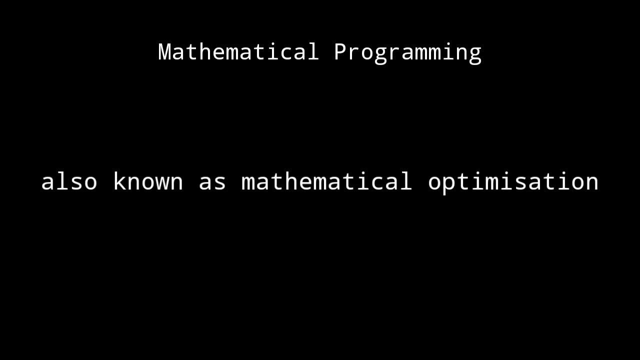 of different theorem-proving strategy. Logical programming languages are mostly used in mathematical proving and predicate calculus. Now we come on to mathematical programming, Now also known as mathematical optimization program. Now it is a selection of the best element from a set of alternatives. Actually, 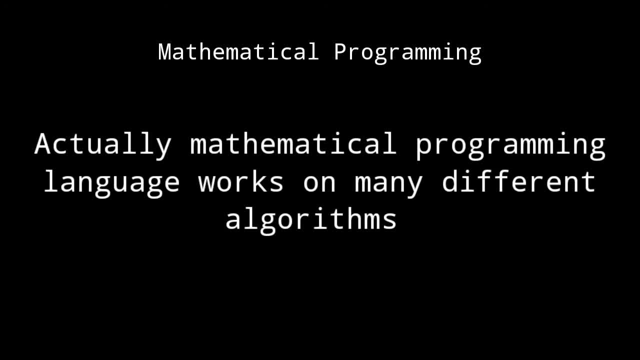 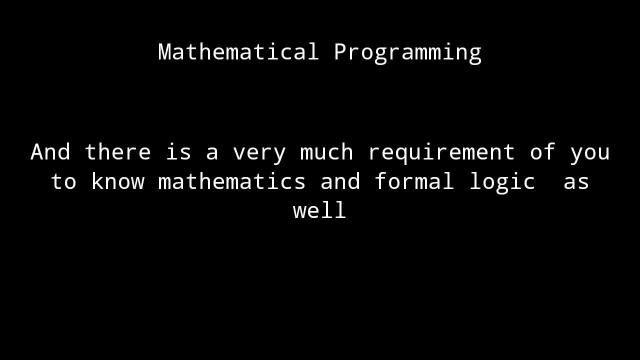 mathematical programming language works on many different algorithms. It may be a kind of linear logic or a concurrent one, And there is a full requirement of you to know mathematics as well as formal logic very well. So I think that's a little bit out of scope. 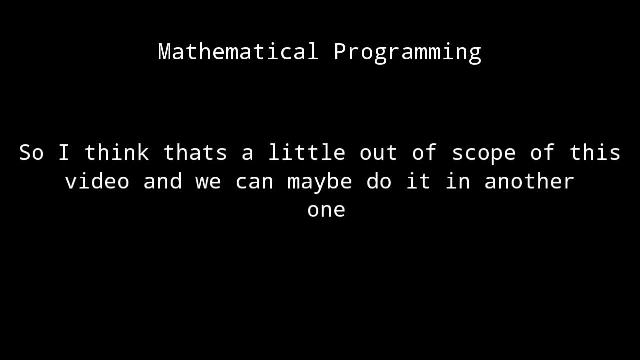 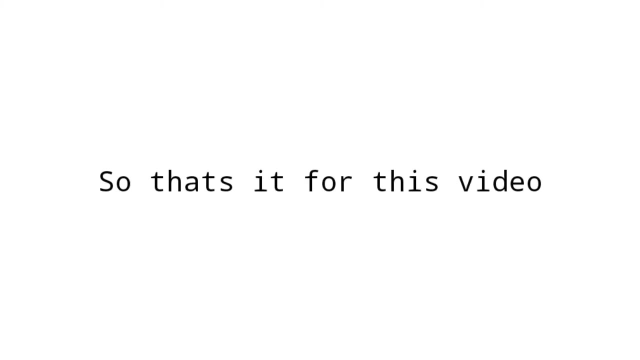 and maybe we can do it in some another video, But it has implementation in economics, mathematics and many other fields, And the best examples exist out there would be OPL, optimization programming language and AMPL. That's it for this video, everyone, And if you liked the video, then hit the like button.